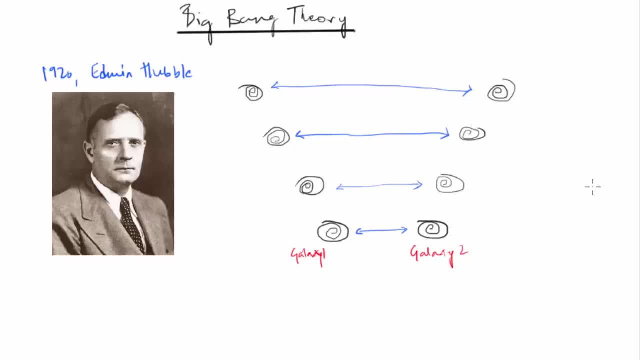 the galaxies is also found to be increasing and thereby the universe is considered to be expanding. But I want you to notice, besides the increase in the distances between the points on the balloon, the points themselves are expanding, But in reality the scientists have no real evidence about the expansion. 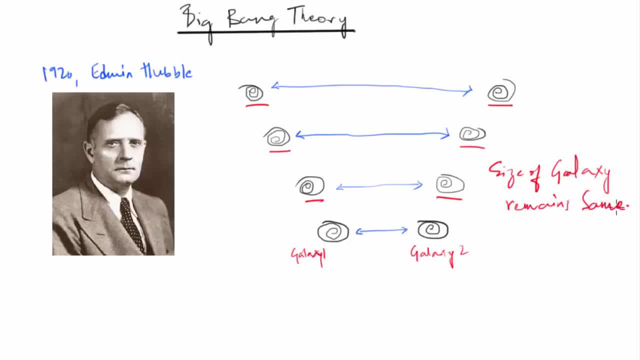 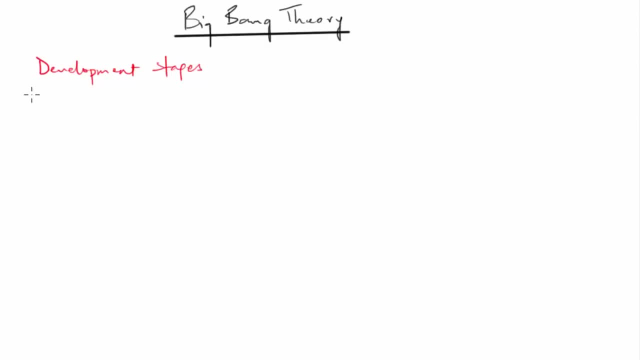 of galaxies, But they do believe that the distance between galaxies is increasing. Hence we can say that the balloon example is only partially correct. Now, the Big Bang Theory considers the following stages in the development of the universe. In the beginning, all matter forming the universe existed in one place, in the form of a tiny balloon. 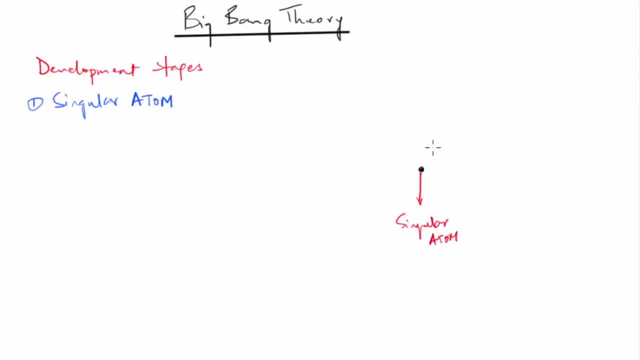 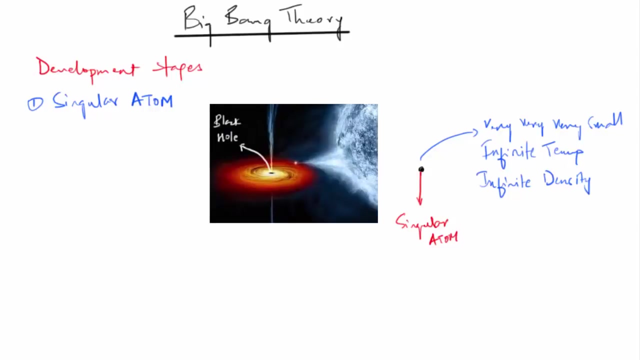 That is, a singular atom with an unimaginably small volume, infinite temperature and infinite density. Well, to be honest, where did it come from? We don't know. Why did it appear? We don't know. It is thought to exist at the core of black holes. Black holes are areas of 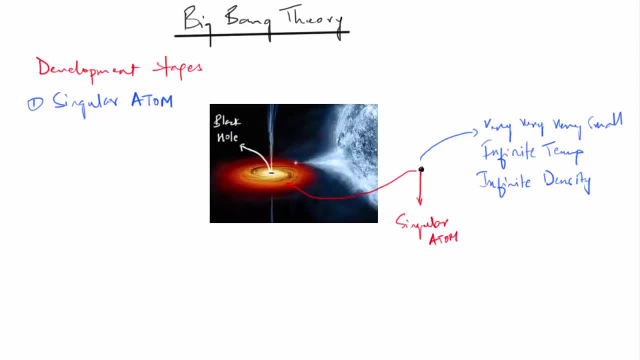 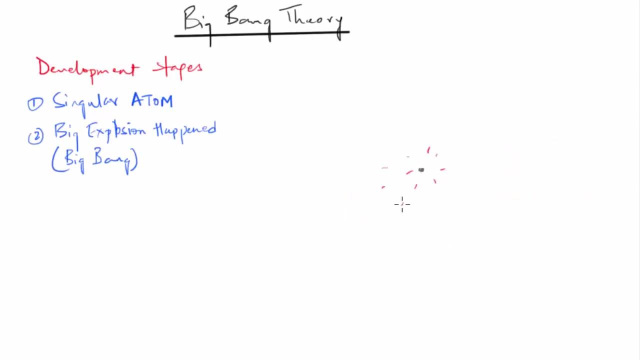 intense gravitational pressure. The pressure is thought to be so intense that finite matter is actually squashed into infinite density. It's a mathematical concept which truly boggles the mind. Now, on the second stage, this tiny ball exploded violently. This led to a huge expansion. The 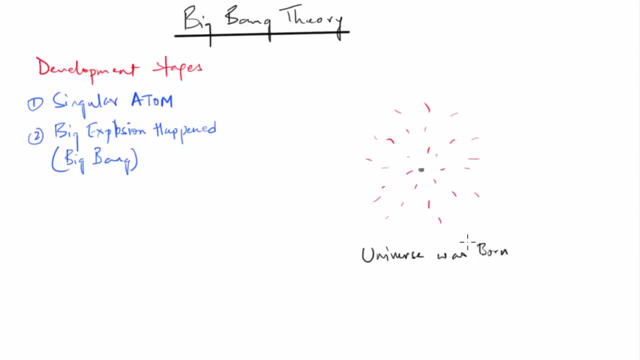 universe that we know was born. Time, space and matter all began with the Big Bang. In a fraction of a second, the universe grew from smaller than a single atom to bigger than a galaxy, And it kept on growing at a fantastic rate. It is still expanding today. 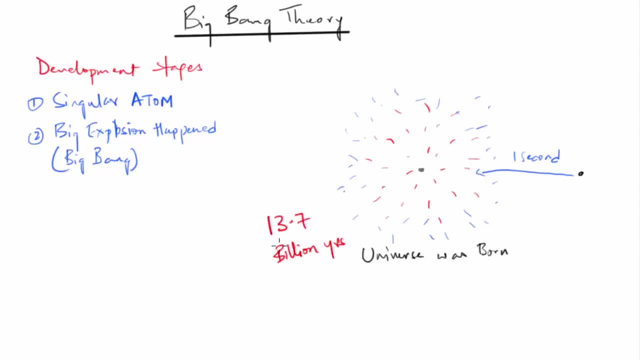 It is now generally accepted that the event of Big Bang- that the universe created in one Big Bang- took place 13.7 billion years before the present. Now, within the first second of the Big Bang, some energy was converted into matter and antimatter. 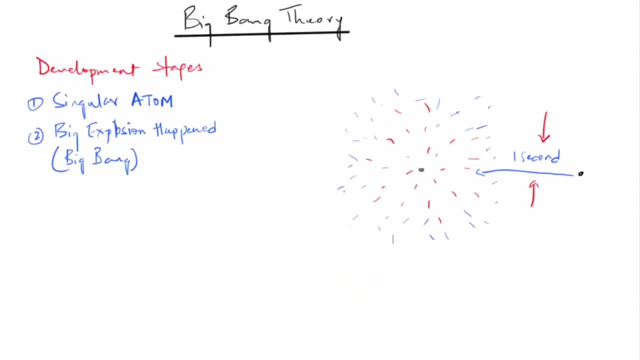 These two opposite types of particle largely destroyed each other, but some matter survived. More stable particles called protons and neutrons started to form. Protons are positively charged and neutrons are negatively charged particles. Over the next 3 minutes, the temperature dropped below 1 billion degree Celsius. 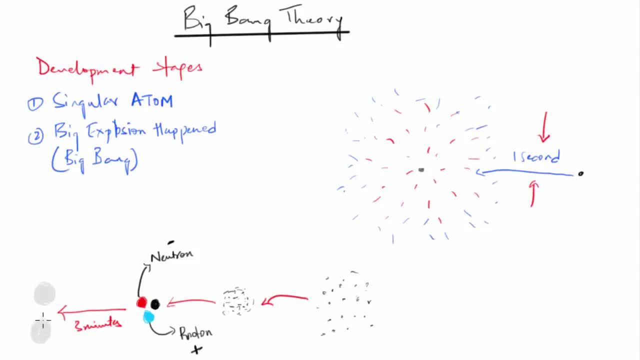 It was now cool enough for the protons and neutrons to come together, basically attract, to form hydrogen and helium nuclei. After 300,000 years, the universe had cooled to about 4000 degrees. Atomic nuclei could finally capture electrons to form a fully fledged atoms.